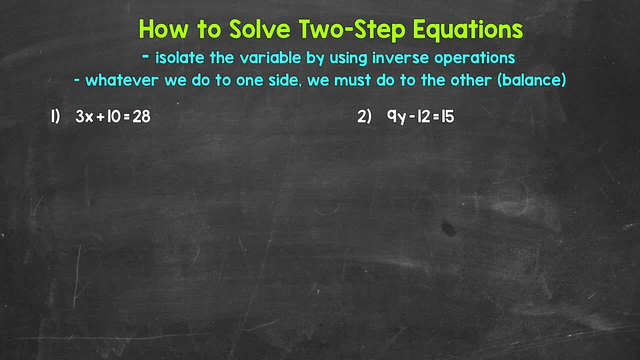 order of operations. here we need to undo the addition first. What's the inverse, The opposite of addition? Well, subtraction. So let's subtract 10 from the left side of the equation. Whatever we do to one side of the equation, we must do to the other, So subtract. 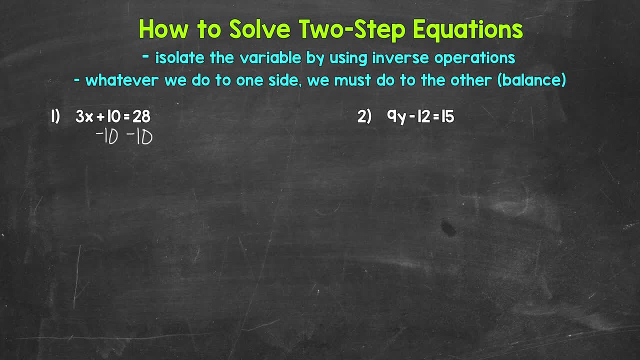 10 from the right side as well. Now, on the left side of the equation, we are adding 10 and subtracting 10.. So these 10s cancel each other out. So we are left with 3x equals. And then on the right side of the equation, we have 28 minus 10, which gives us 18.. 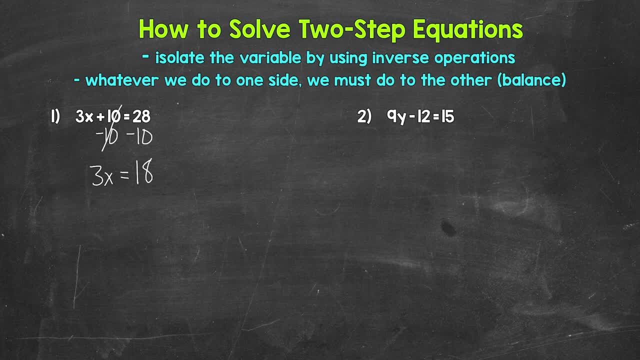 So now we have: 3x equals 18.. We are multiplying x by 3. So we need to undo that. We need the inverse operation here in order to isolate x. The inverse operation of multiplication is division. Let's divide the left side of the equation by 3.. Whatever we do to one side, we must do to the. 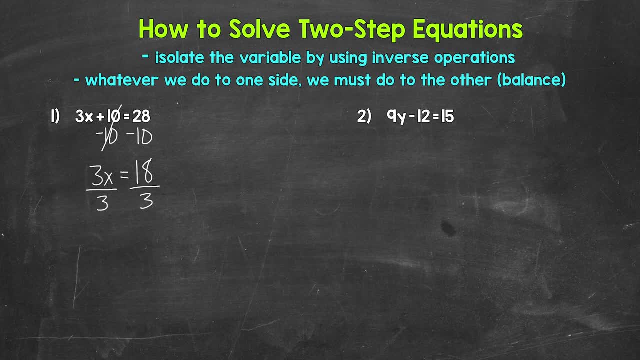 other. So divide the right side by 3 as well. On the left side of the equation we are multiplying by 3 and dividing by 3.. So these 3s cancel each other out. Now our variable x is isolated, So we: 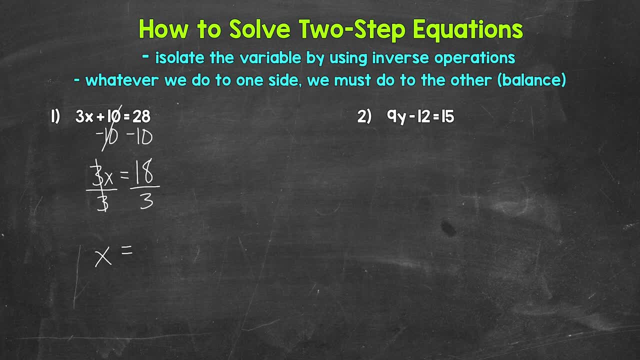 have x equals And then on the right side of the equation, we are multiplying x by 3.. So we need to. that's our solution. Now, one last thing we can do: we can always check to see if we are correct, And we do that by plugging in what we got and seeing if it works. So, for example, let's plug in: 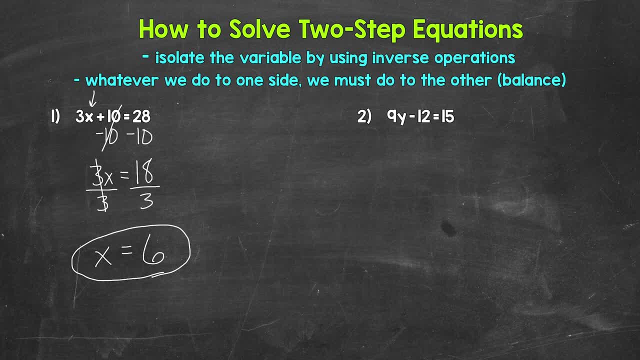 6 for x and see if it works. So we can come to the side here. 3 times 6 plus 10 equals 28.. So we need to multiply first. 3 times 6 is 18.. So we have 18 plus 10.. 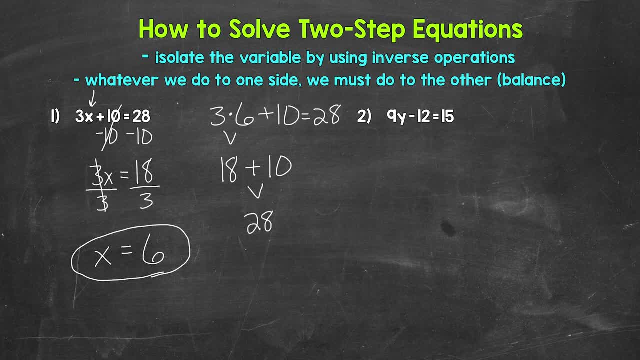 18 plus 10 is 28.. So we are correct: X equals 6.. Let's move on to number 2, where we have 9y minus 12 equals 15.. So 9 times what minus 12 equals 15.. 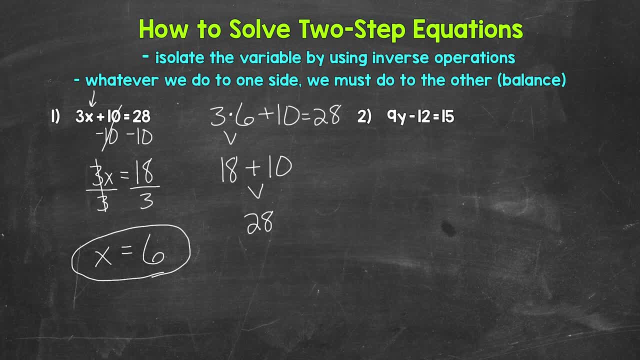 We need to isolate that variable of y. We need to undo the operations. on that side of the equation We have multiplication and subtraction, So we need to go in the reverse order of operations in order to undo everything here. We need to undo the subtraction first. 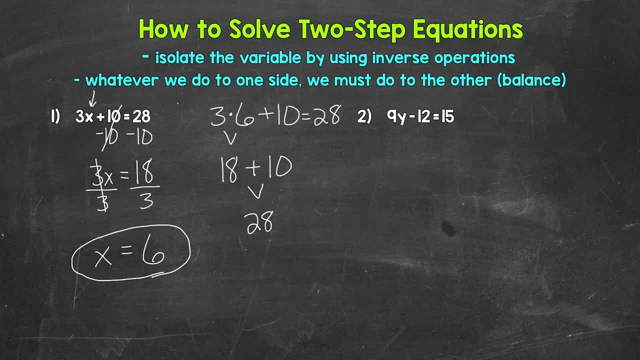 So what's the inverse operation of subtraction? Well, addition. So let's add 12 to the left side of the equation. Whatever we do to one side, we must do to the other. So add 12 to the right side as well. 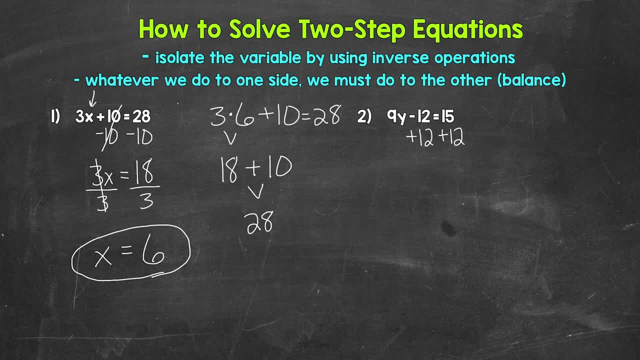 On the left side, we are subtracting 12 and adding 12.. So these 12s cancel each other out. So we have 9y equals. And then on the right side of the equation, 15 plus 12 gives us 27.. 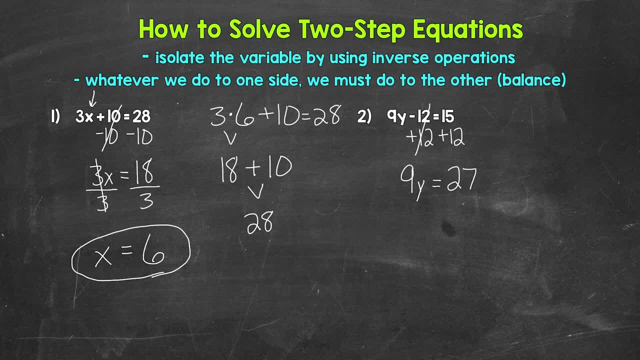 So now we have 9y equals 27.. So we're multiplying y by 9 and we need to undo that multiplication by using the inverse operation. What's the inverse operation of multiplication? Well, division. So let's divide the left side by 9.. 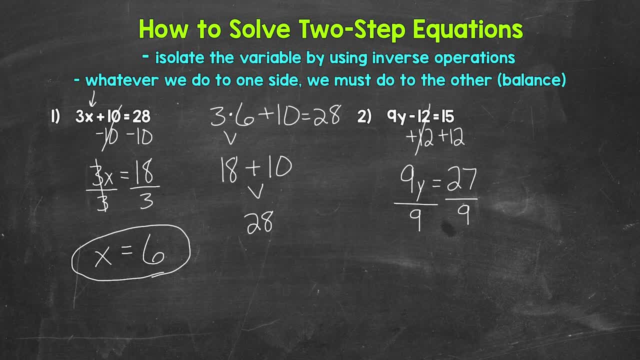 Whatever we do to one side, we must do to the other. So division. So let's divide the right side by 9 as well. On the left side, we are multiplying by 9 and dividing by 9.. So these 9s cancel each other out. 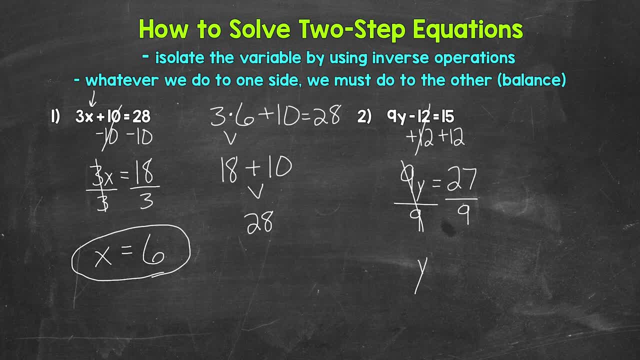 And our variable y, is now isolated. So we have y equals. And then on the right side of the equation we have 27 divided by 9, which gives us 3. So y equals 3. And that's our solution. 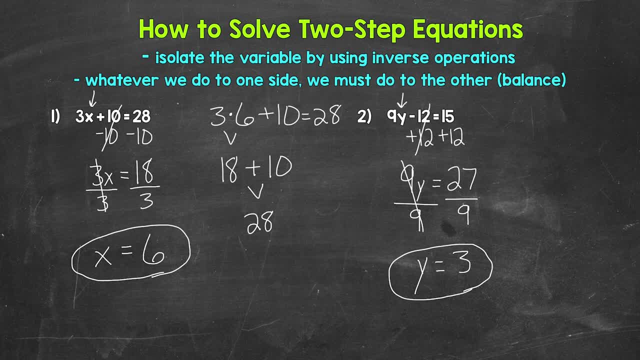 Now let's do the inverse operation. Let's plug it in and see if we are correct. So plug in 3 for y. So 9 times 3 minus 12 equals 15.. So we start with multiplication: 9 times 3 is 27.. 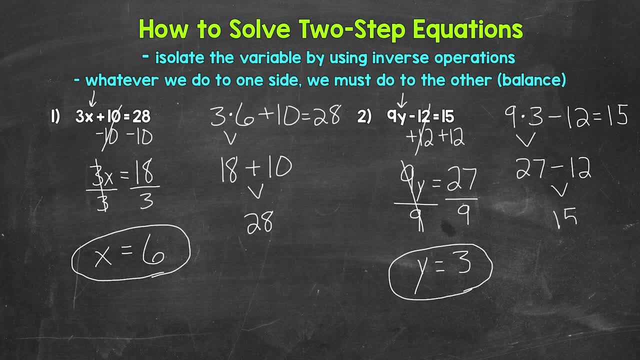 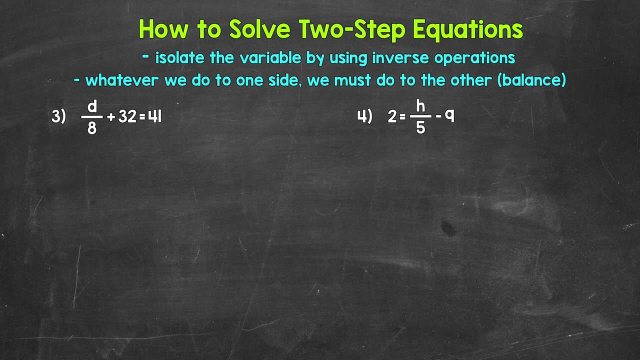 27 minus 12 is 15.. So we are correct: y equals 3.. Let's move on to Numbers 3 and 4.. So here are numbers 3 and 4.. Let's jump into number 3, where we have: d divided by 8 plus 32 equals 41.. 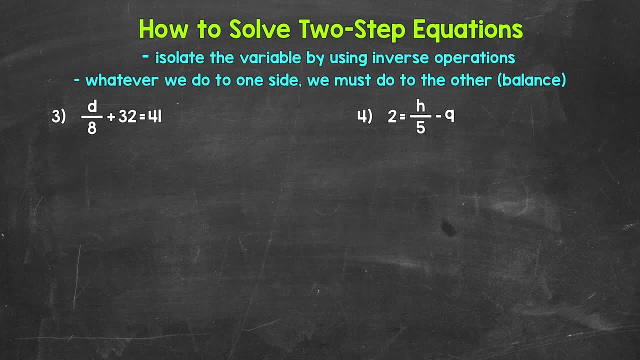 So we need to isolate that variable of d using inverse operations And we need to go in the reverse order of operations. We need to undo the addition first. So what's the inverse operation of addition? Well, Subtraction. So let's subtract 32 from the left side of the equation. 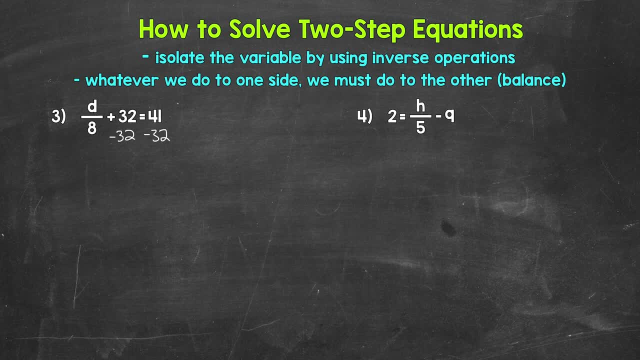 Whatever we do to one side, we must do to the other. So subtract 32 from the right side as well. Now, on the left side of the equation, we are adding 32 and subtracting 32.. So these 32s cancel each other out. 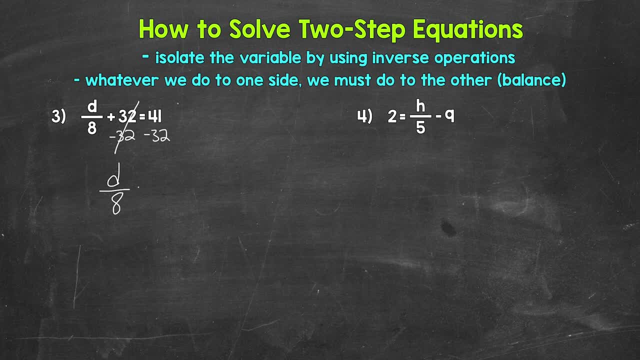 So we have d divided by 8, equals. And then on the right side, On the left side of the equation, we have 41 minus 32.. That gives us 9.. So we have d divided by 8 equals 9.. 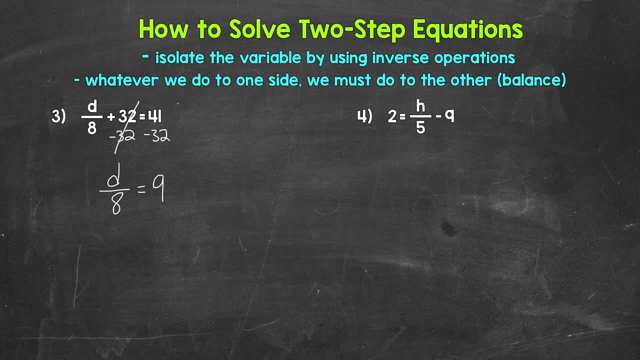 So let's continue to look to isolate that variable of d. So d is being divided by 8. What's the inverse operation, The opposite of division? Well, multiplication. So let's multiply the left side by 8.. Whatever we do to one side. 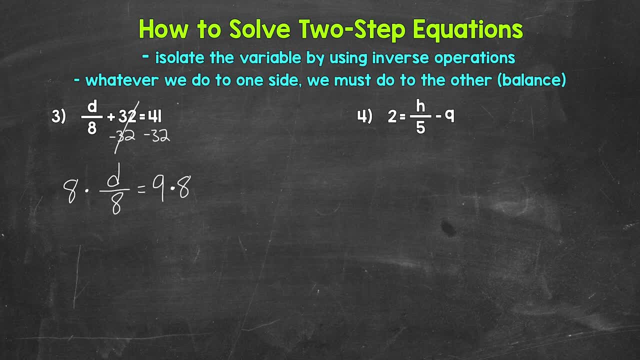 We must do. We must do to the other. So multiply the right side by 8 as well. Now, on the left side, we are dividing by 8 and multiplying by 8. These 8s cancel each other out. So d is now isolated. 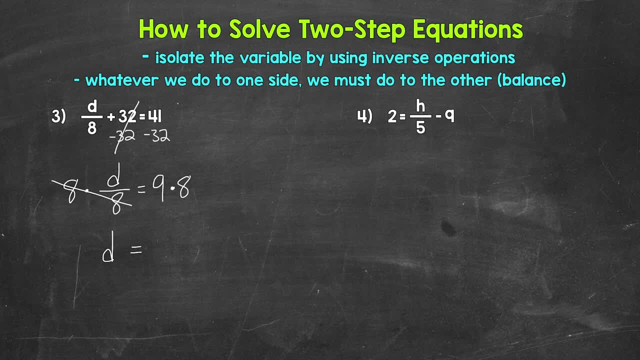 d equals. And then, on the right side, 9 times 8 gives us 72.. So d equals 72.. That's our solution. And let's check that by plugging 72.. 72 in 4d, So we have 72 divided by 8 plus 32 equals 41. 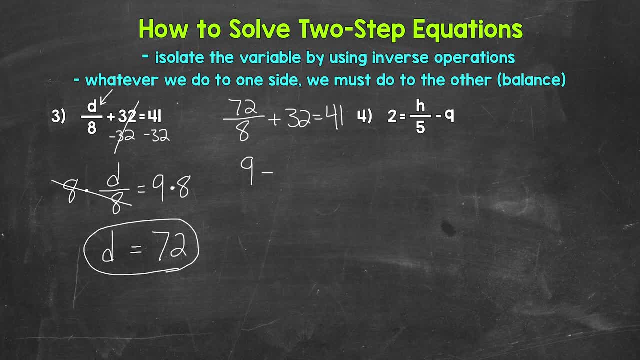 72 divided by 8 is 9.. So we have 9 plus 32.. And that gives us 41. So we are correct, d equals 72.. Lastly, let's move on to number 4.. Where we have: 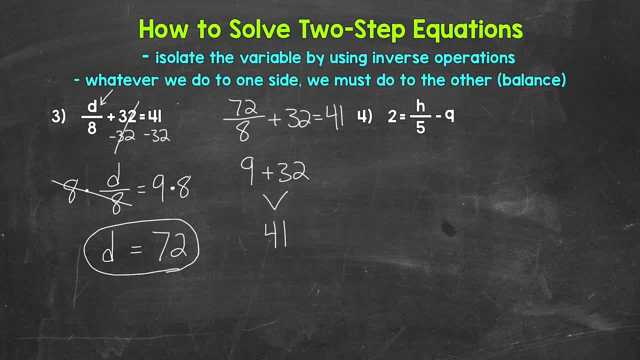 2 equals h divided by 5 minus 9.. Now for number 4, the variable is on the right side of the equation, So a little bit of a different look here, But we use the same exact process, So this doesn't change anything. 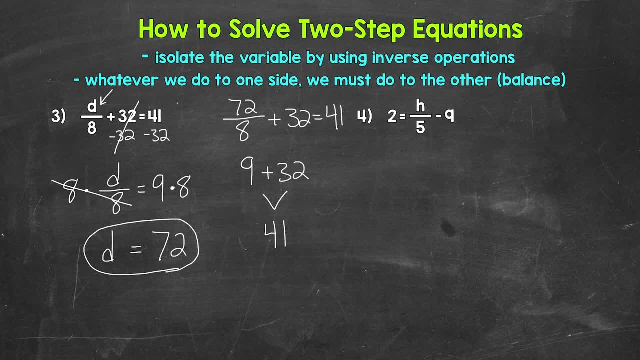 So we need to isolate that variable of h. So h is being divided by 5. And then we are subtracting 9. So let's undo that subtraction first. What's the inverse? What's the inverse operation of subtraction? Well, addition. 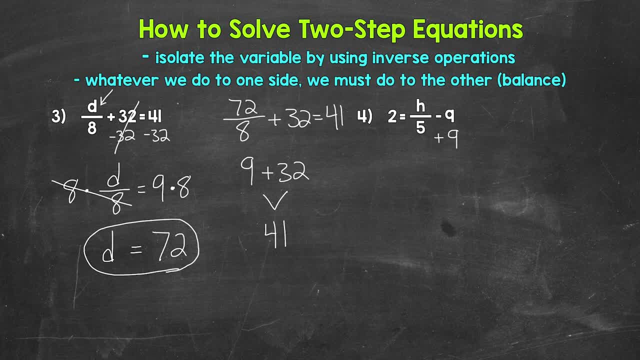 So let's add 9 to the right side of the equation. That means we need to add 9 to the left side as well. Now, on the right side of the equation, we are subtracting 9 and adding 9.. So those 9s cancel each other out. 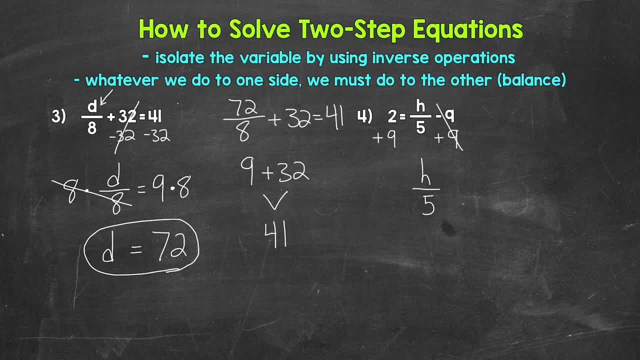 So we have h divided by 5 equals, And then on the left side we have 9.. And then on the right side, 2 plus 9 gives us 11.. So h divided by 5 equals 11.. So we are dividing h by 5.. 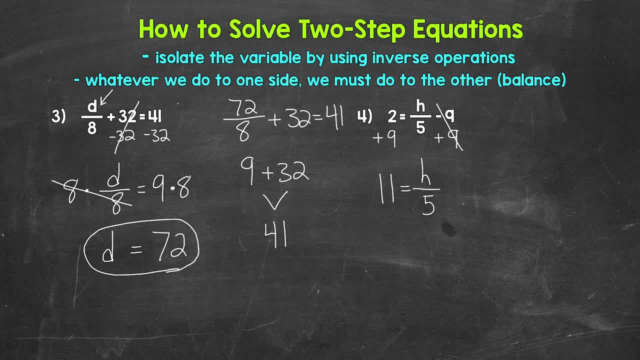 What's the inverse operation of division? Well, multiplication. So let's multiply the right side by 5.. That means we need to multiply the left side by 5 as well. Now, on the right side of the equation, we are dividing by 5.. 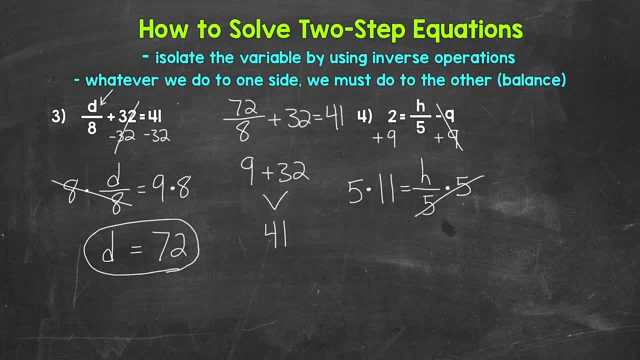 And multiplying by 5.. So these 5s cancel each other out And h is now isolated. So we have h equals. And then, on the left side of the equation, 5 times 11 gives us 55. So h equals 55.. 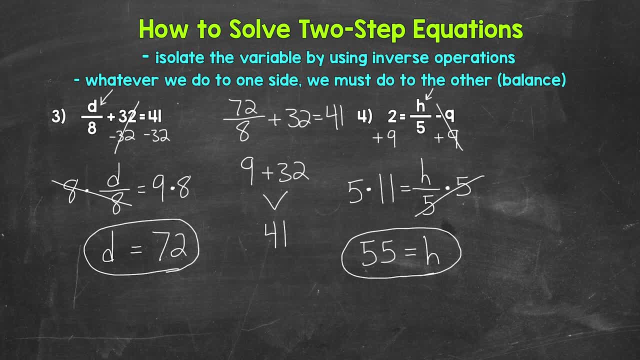 So that's our solution. And let's check it by plugging 55 in for h. So 2 equals 55.. So h equals 55 divided by 5 minus 9.. 55 divided by 5 is 11.. And 11 minus 9 is 2.. 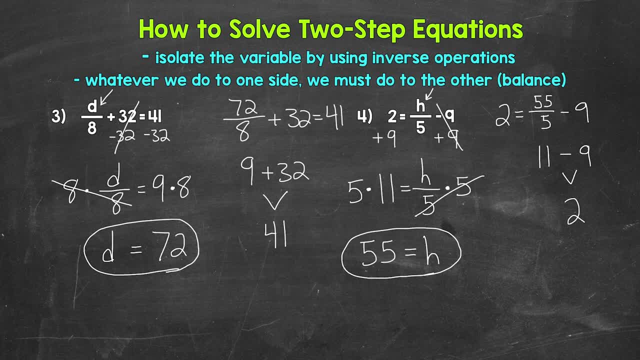 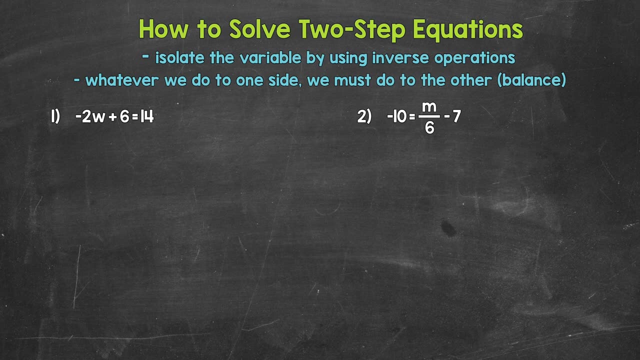 So we are correct: h equals 55. So there are our four introductory examples. Let's move on to a couple of examples involving negatives. Here are our examples involving negatives. Here are our examples involving negatives, involving negatives. Let's jump into number one, where we have 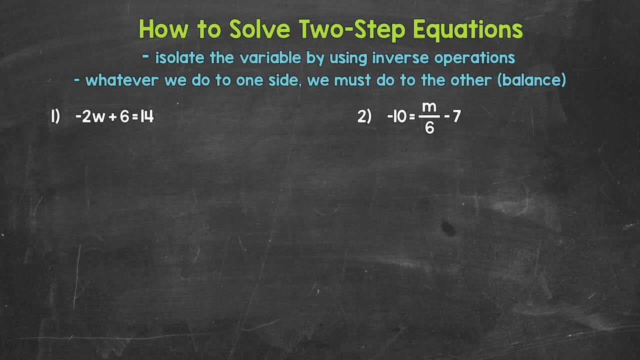 negative two w plus six equals 14.. So negative two times what plus six equals 14.. We need to isolate that variable of w by using inverse operations And we will go in the reverse order of operations. So we need to undo the addition first. 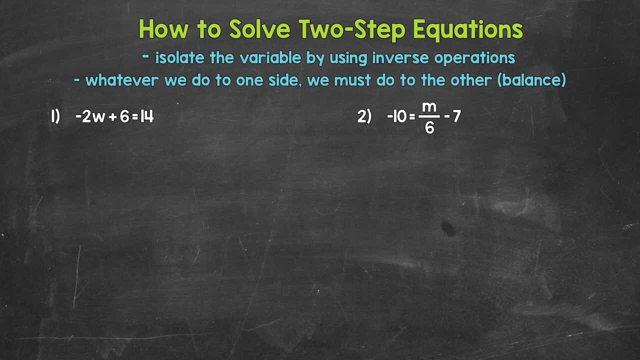 What's the inverse operation of addition, Subtraction. So we need to subtract six from the left side of the equation. Whatever we do to one side of the equation, we must do to the other. So subtract six from the right side as well. 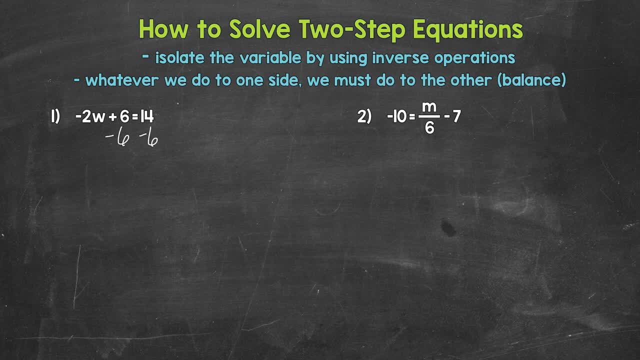 Now on the left side of the equation we are adding six and subtracting six, So these sixes cancel each other out. So we have negative two times negative, two w equals. and then on the right side of the equation, 14 minus six. 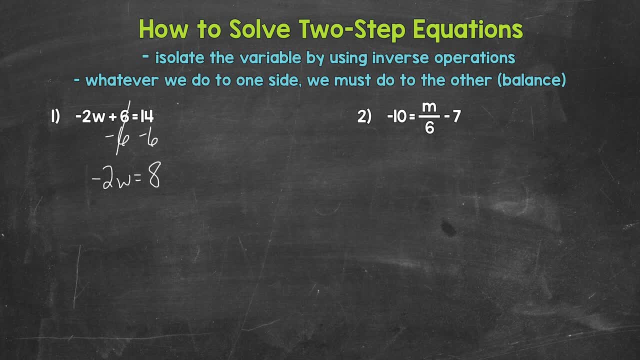 That gives us eight. So we have negative two. w equals eight now. So we are multiplying w by negative two. We need to undo that multiplication. What's the inverse operation of multiplication? Well, division. So let's divide the left side of the equation. 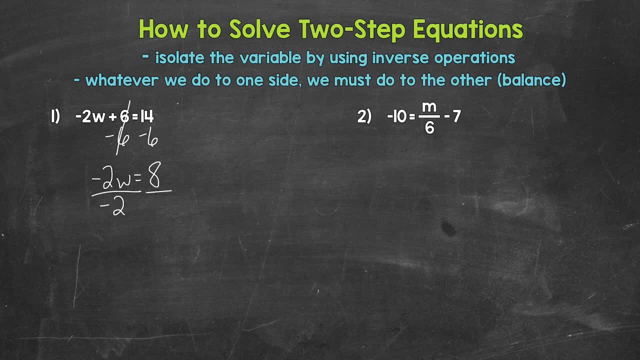 We need to divide the right side of the equation by negative two. Whatever we do to one side, we must do to the other. So divide the right side by negative two as well. Now, on the left side of the equation, we are multiplying by negative two. 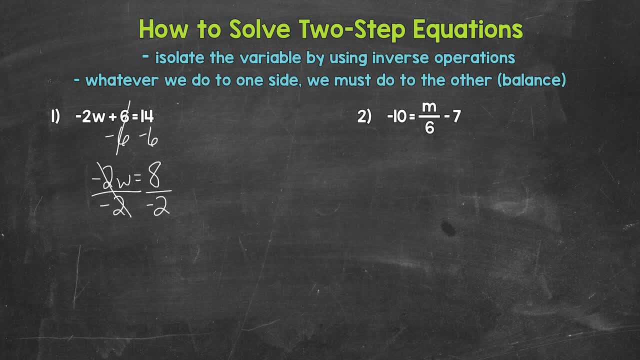 and dividing by negative two. So these negative twos cancel each other out. W is now isolated, So we have w equals. and then on the right side of the equation we have eight divided by two. So we have a positive, positive, eight divided by a negative. 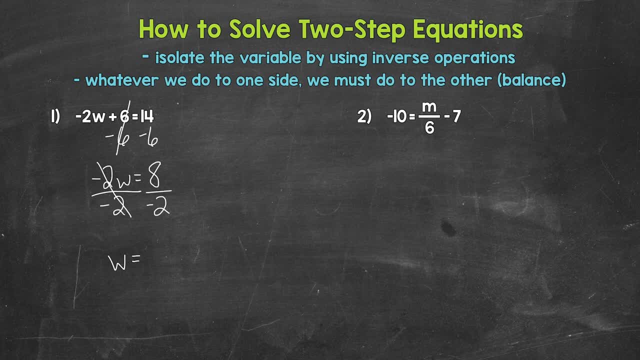 negative two. When we divide a positive by a negative, we get a negative. So eight divided by negative two gives us negative four. So we need to be careful there. when we have negatives involved, W equals negative four, And that's our solution. 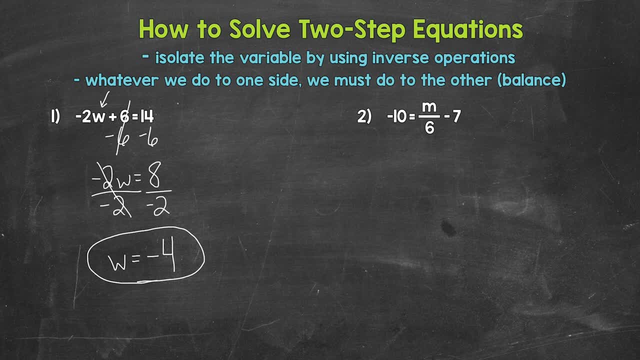 Now we can check this by plugging negative four in for w and seeing if it works. So let's do that. So we have negative two. let's come to the side here. times negative four plus six equals 14.. All right, let's start with multiplication. 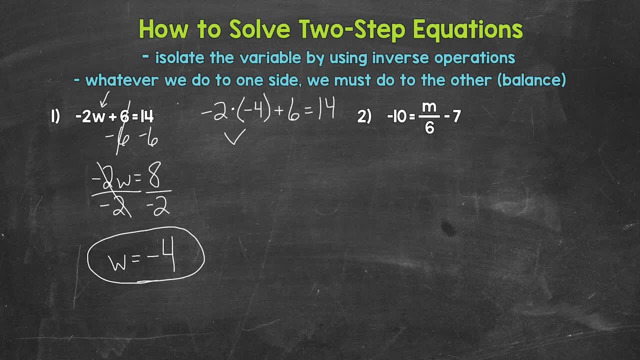 So we have negative two times negative, four a negative times a negative equals a positive, a negative times a negative equals a positive. a negative times a negative equals a positive. so this gives us eight, And then we have eight plus six, which is 14.. 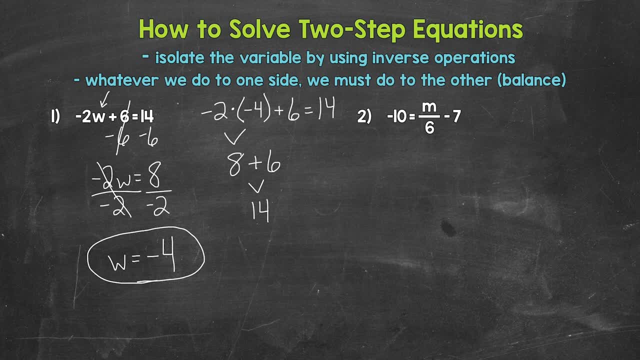 So we are correct. W equals negative four. Let's move on to number two, where we have negative 10 on the left side of the equation equals, and then on the right side we have m divided by six minus seven. So what divided by six minus seven equals? 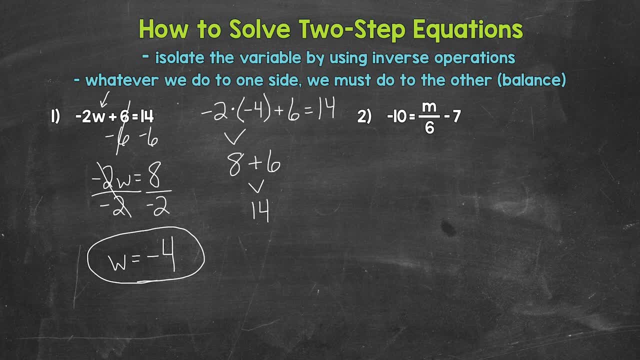 negative 10.. So we need to look to isolate that variable of m. So, taking a look at that side of the equation, we need to undo the subtraction first, So we have minus seven. What's the inverse operation of subtraction? Well, addition. 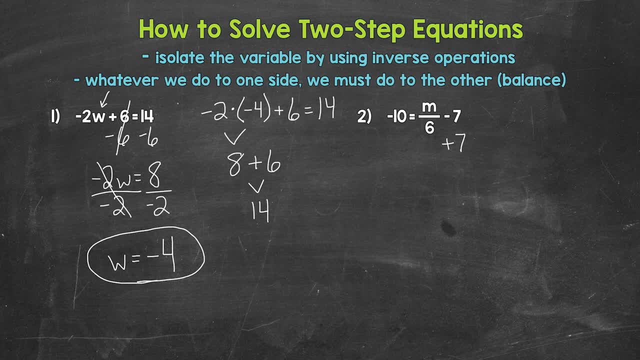 So let's add seven to the right side of the equation. Whatever we do to one side, we must do to the other. Now, on the right side of the equation, we are subtracting seven and add seven again and adding 7.. So these 7s cancel each other out. So now we have m divided by 6. 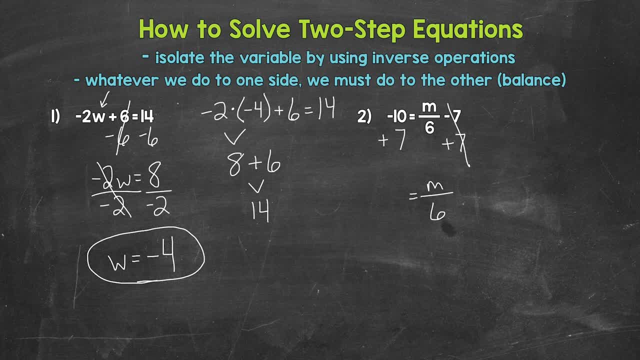 equals. and then on the left side of the equation we have negative 10 plus 7. So we are starting at negative 10, and we are adding a positive 7. So we are increasing in value by 7. That gives us. 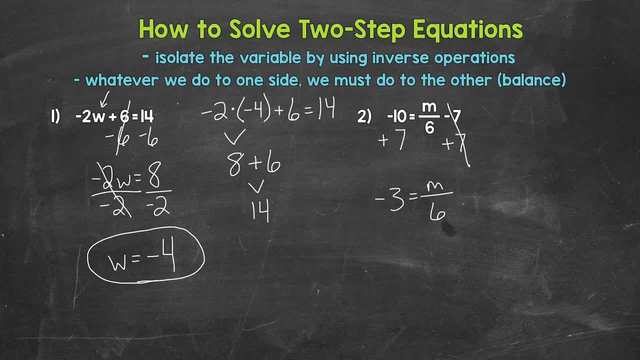 minus negative 3.. So now we have m divided by 6 equals negative 3.. So let's isolate that variable of m. We are dividing m by 6.. So what's the inverse operation of division? Well, multiplication. So let's multiply that side of the equation by 6.. Whatever we do to one side of the equation, 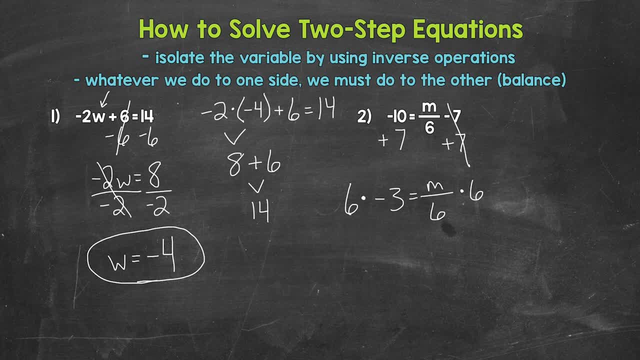 we must do to the other. So multiply the left side by 6, as well. Now on the right side of the equation we are dividing by 6 and multiplying by 6.. So these 6s cancel each other out. m is now isolated, So we have m equals. and then on the left side of the 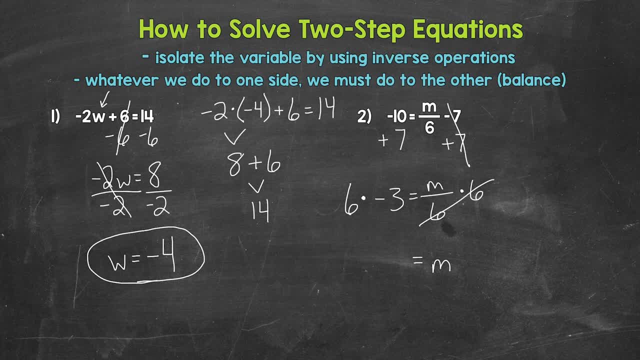 equation: 6 times negative, 3.. Well, we have a positive times a negative, A positive times a negative. gives us a negative. So 6 times negative, 3. gives us negative 18.. So m equals negative 18.. And that's our solution. Let's check it by plugging. 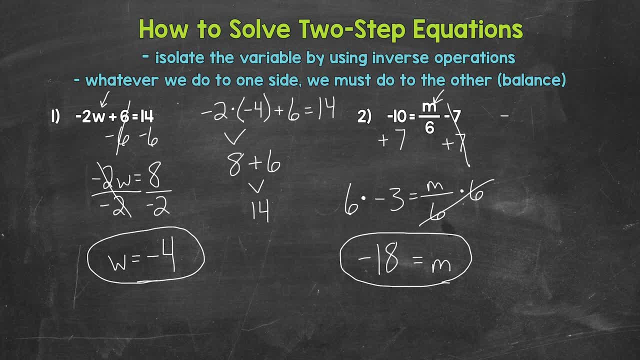 negative 18 in for m. So we have: negative 10 equals negative 18 divided by 6 minus 7.. Let's start with division. So we have negative 18 divided by 6,. a negative divided by a positive equals a negative, So that gives us negative 3.. And now we have: 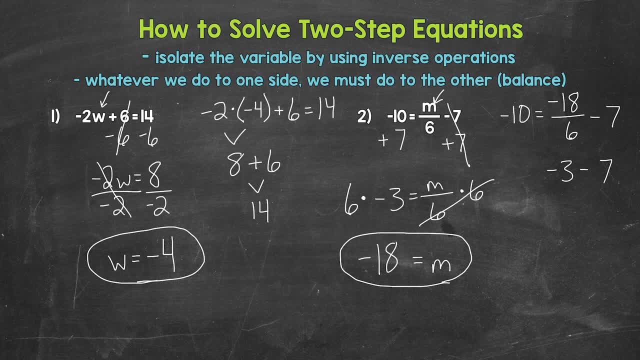 negative 3 minus 7.. Now there are a couple different ways to think through this. So we are starting at negative 3 and subtracting 7. So we are decreasing in value by 7. That gives us negative 10.. Another way to think through this: whenever we have subtraction, we can: 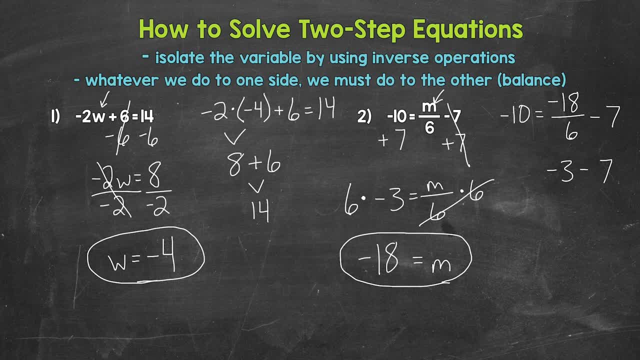 add the opposite, And that will give us the correct answer as well. So add the opposite. So we have negative 3 plus negative 7. That gives us negative 10 as well. So we are correct: m equals negative 18.. So there you have it. There's how to solve two-step equations involving 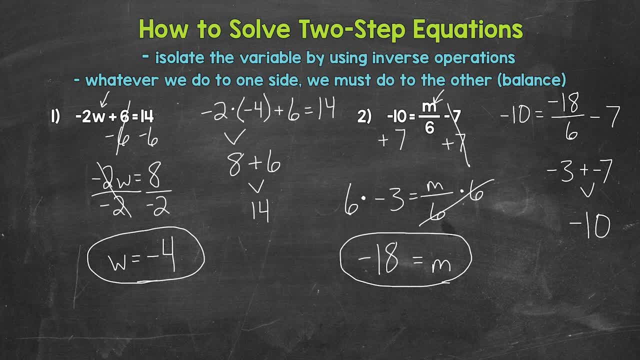 negatives. Just keep in mind, be careful when working with those negatives And if you need more help or examples, please let me know in the comments. Thank you so much for watching. with addition, subtraction, multiplication or division involving negatives, I added links to: 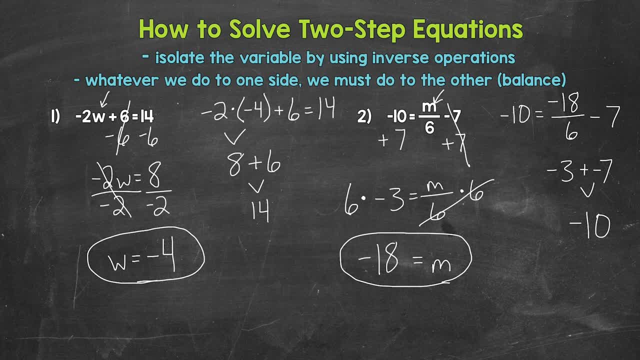 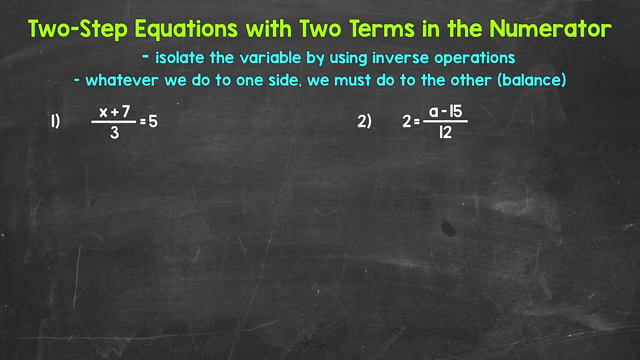 those videos down in the description. So there are our examples involving negatives. Let's move on to equations with two terms in the numerator. Here are our examples with two terms in the numerator. So basically, one side of the equation is set up in fractional form. Let's jump into 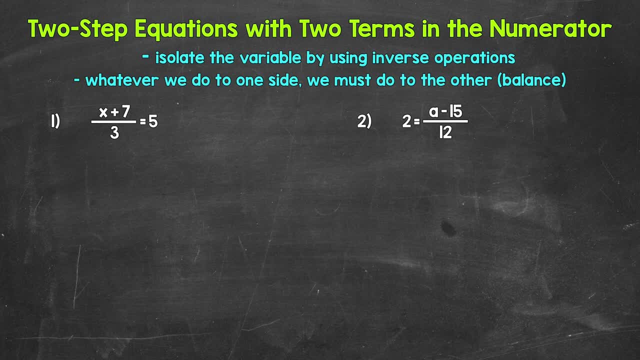 number one, where we have x plus 7 as our numerator and 3 as our denominator, equals 5.. So something plus 7 divided by 3 equals 5.. Remember, when we are set up in fractional form, we have that fraction bar. That means we are dividing. Now we're not just dividing x by 3 or 7 by 3.. We can. 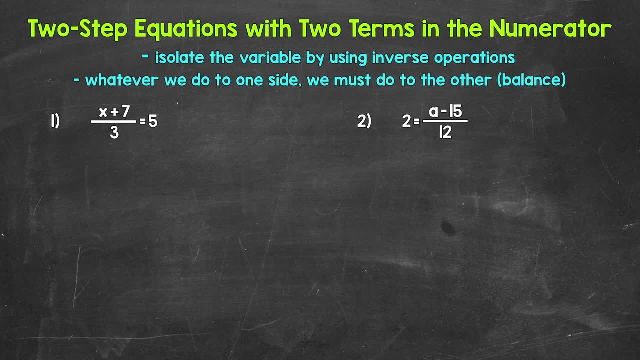 think of that fraction bar as a grouping symbol. x plus 7 is being divided by 3. We can even put parentheses here to group the numerator. Again, that fraction bar acts as a grouping symbol And we divide the numerator by the denominator. 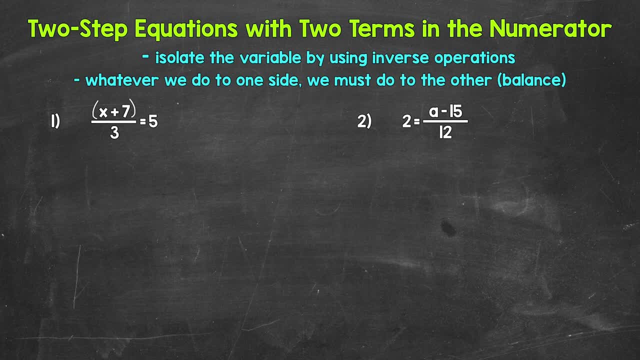 Now we need to isolate that variable of x by using inverse operations, And we're going to go in the reverse order of operations. We have addition and division here, But the addition is grouped. It's in parentheses, So we're going to go in the reverse order of operations. 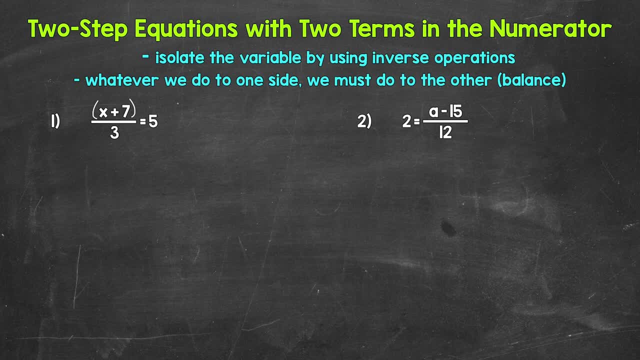 And then we have division. We need to undo the division first, So we can think of this as getting rid of the fraction first. So what's the inverse operation of division? Well, multiplication. So let's multiply the left side of the equation by 3.. Whatever we do to one side, we must do to the. 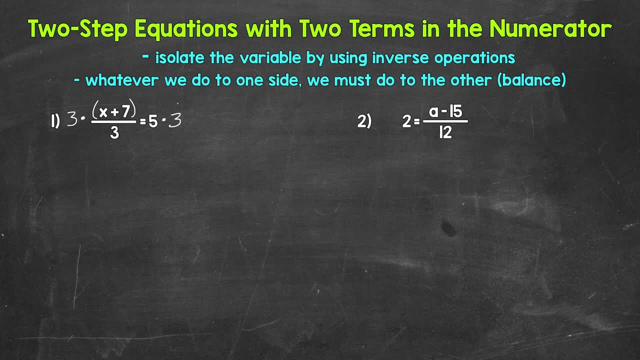 other. So multiply the right side by 3 as well. Now on the left side we are dividing by 3. So we're multiplying by 3. So these 3s cancel each other out. Now we just have x plus 7 on the left side. 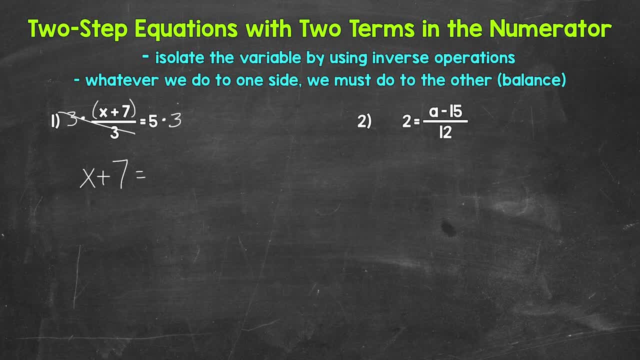 equals. And then, on the right side, 5 times 3 gives us 15.. And now we have x plus 7 equals 15.. So we are adding 7 to x. We need to undo that addition in order to isolate the variable. What's the? 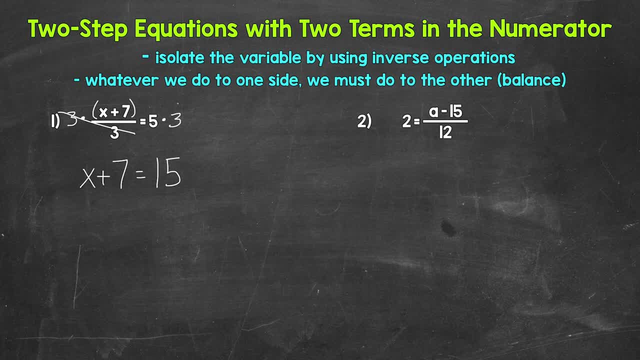 inverse operation of addition, Well, subtraction. So let's subtract 7 from the left side. Whatever we do to one side, we must do to the other. So subtract 7 from the right side as well. On the left side of the equation we are. 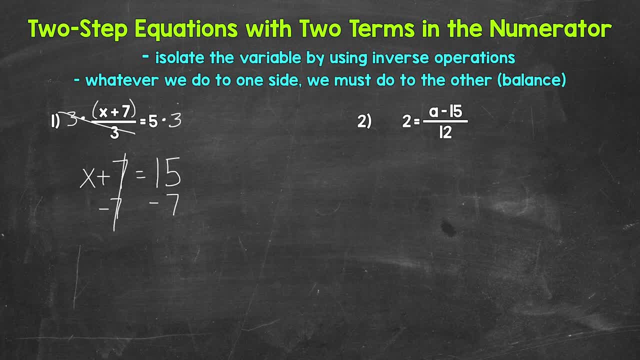 adding 7 and subtracting 7.. So these 7s cancel each other out. x is now isolated, So we have x equals. And then on the right side, 15 minus 7 gives us 8. So we have x plus 7.. And then, on the 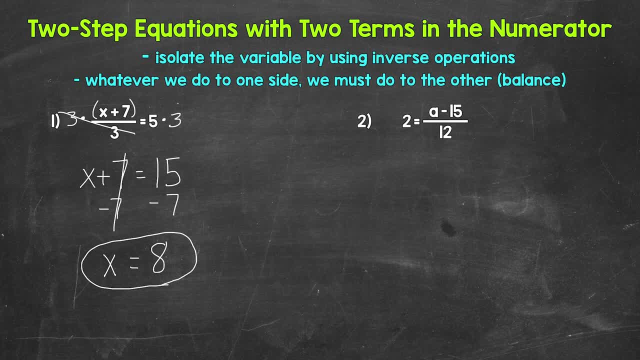 left side: 15 minus 7 gives us 8.. x equals 8. And that's our solution. Now we can check that by plugging 8 in for x and seeing if it works. So let's come to the side. We have 8 plus 7 divided. 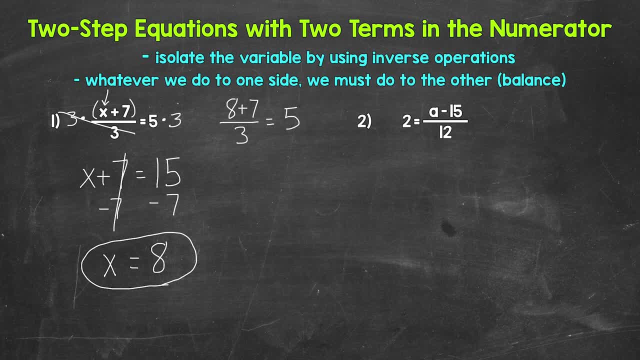 by 3 equals 5.. So let's start with our numerator: 8 plus 7.. Remember that fraction bar acts as a grouping symbol, So we will work through the numerator and then the denominator. So let's divide: 8 plus 7 is 15.. So we have 15 divided by 3. That does give us 5. So we are correct x. 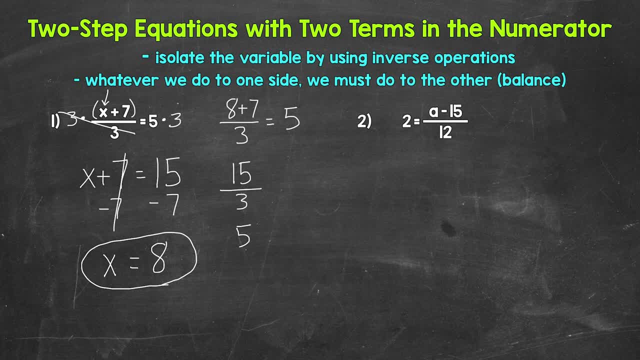 equals 8.. Let's move on to number 2, where we have 2 on the left side of the equation equals, and then on the right side of the equation, a minus 15 divided by 12.. We have subtraction and division, But the subtraction is not the same as the division. So we have subtraction and 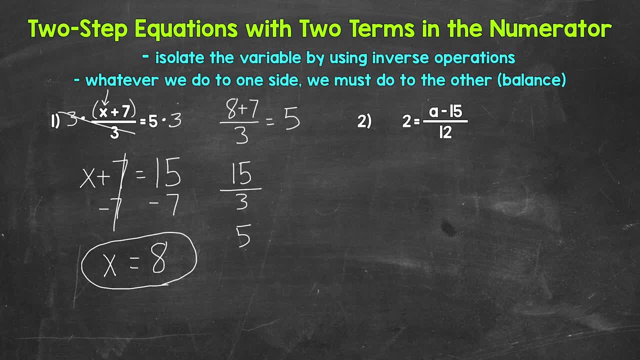 division, But the subtraction is grouped in the numerator And we can even use parentheses to help us picture that. We don't have to write those parentheses, but it is an option. So we need to undo the division first. We need to get rid of the fraction. So what's the inverse operation? 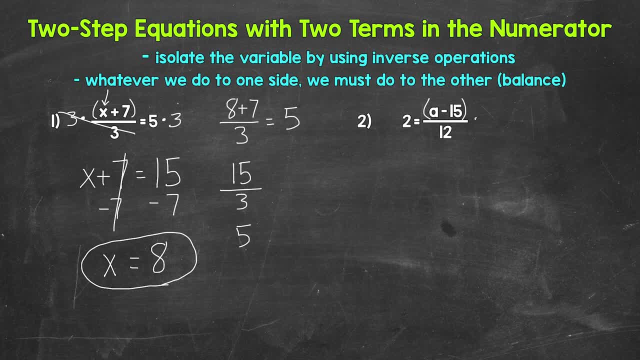 of division? Well, multiplication. So let's multiply the right side by 12.. Whatever we do to one side, We must do to the other. So multiply the left side by 12 as well. On the right side, we are dividing by 12 and multiplying by 12. These 12s cancel each other out, So now we just have a minus. 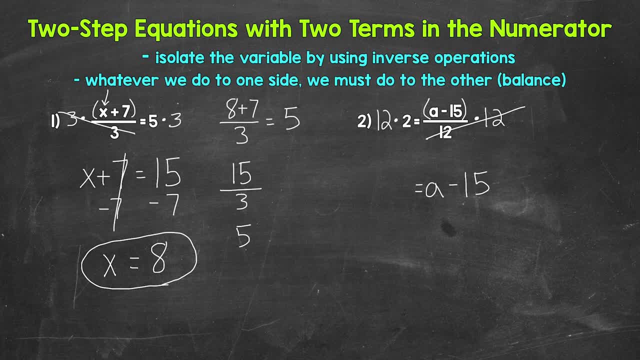 15 equals, and then on the left side, 12 times 2 gives us 24.. So a minus 15 equals 24.. We are subtracting 15 from A, So we need to undo that subtraction. What's the inverse operation of? 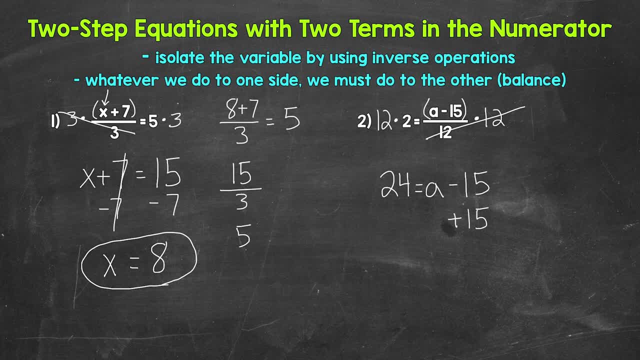 subtraction, Well, addition. So let's add 15 to the right side. Whatever we do to one side, we must do to the other. So add 15 to the left side as well. On the right side we are subtracting 15. 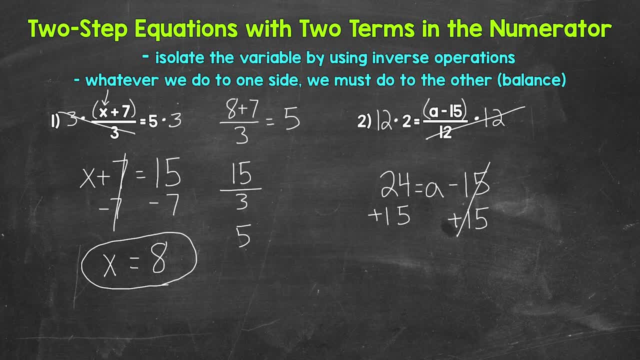 and adding 15.. So the 15s cancel each other out. A is now isolated, So we have 15 plus 15.. So we have A equals. And then on the left side, 24 plus 15 gives us 39. So A equals 39. That's our. 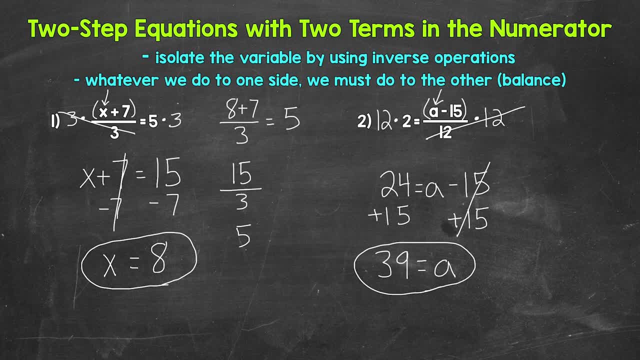 solution, And we can check it by plugging 39 in for A. So let's come to the side here. 2 equals 39 minus 15 divided by 12.. Let's start with the numerators. So we have 39 minus 15.. That gives us 24.. And now we have 24 divided by 12,. 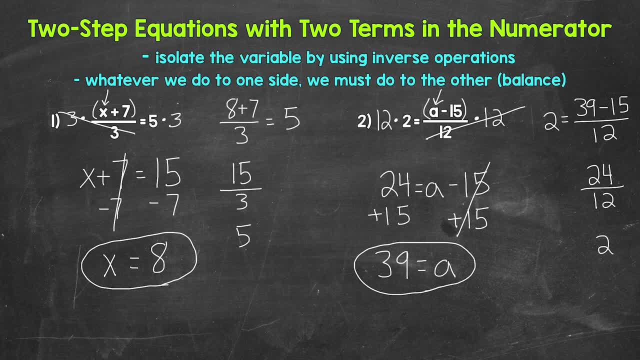 which does give us 2.. So we are correct. A equals 39.. So there you have it. There's how to solve two-step equations. I hope that helped. Thanks so much for watching. Until next time, peace.